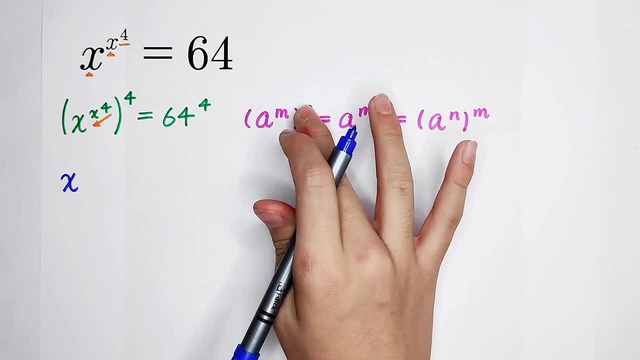 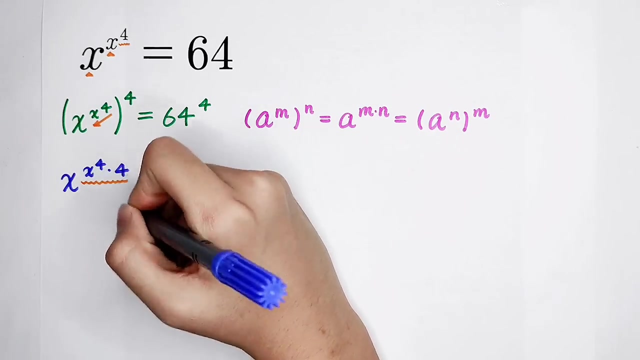 and n is this 4.. So it is m, then times n. It is x. to the power of x, to the power of 4, then times 4.. So this is the new exponent. The right-hand side is still 64, and then to the power of 4.. 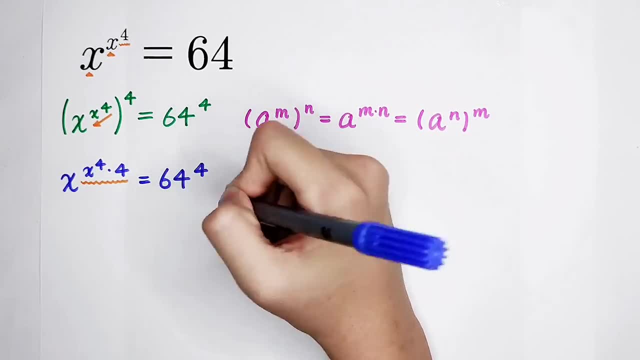 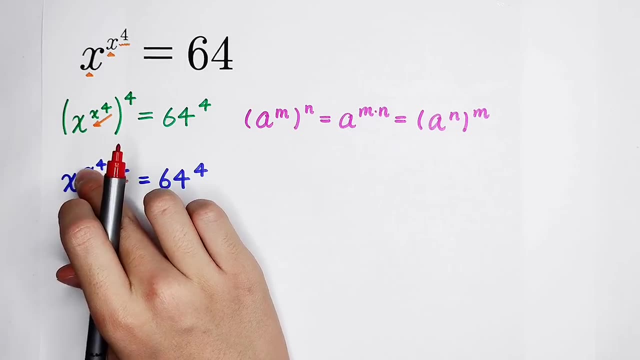 Use this formula: n is 4.. m is x to the power of 4. So it is equal to h to the power of n and then all to the power of m And a. is this x on the bottom? So it is equal to. 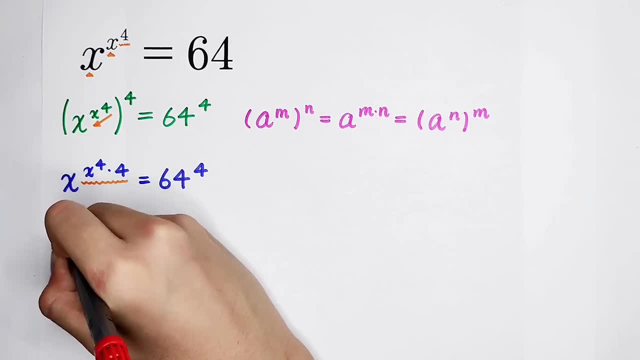 x to the power of m, and then all to the power of m. So it is x to the power of 4.. And then all to the power of x. to the power of 4. It is equal to 64, and then all to the power of 4.. 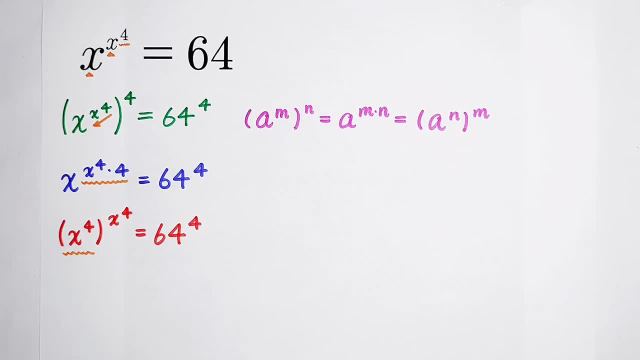 The base is x to the power of 4.. And the exponent is also x to the power of 4.. They have the same value, So it becomes the form of something to the power of itself. Now I have a hopeless- I hope- the right-hand side. 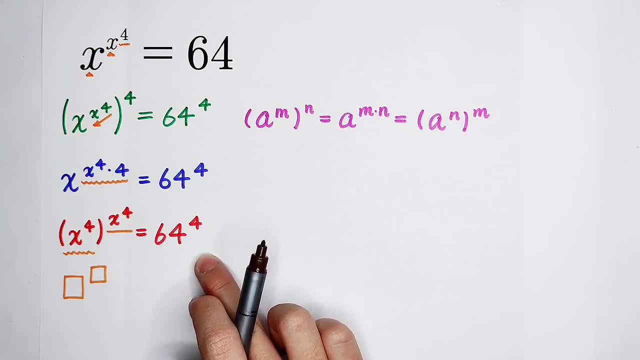 64 to the power of 4, can be also written into the form: something to the power of itself, Now, because 64 is a nice number. it is 8 squared. So 64 then, to the power of 4,. it can be written as: 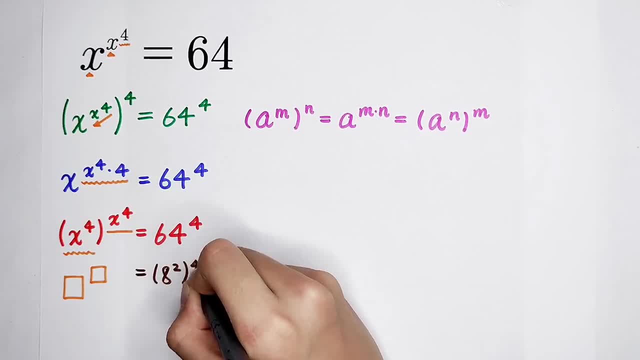 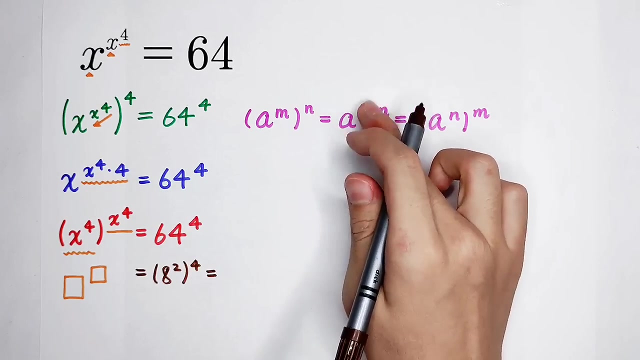 8 squared, and then all to the power of 4.. So use this formula: a is 8,, m is 2, and n is 4.. So it is equal to a to the power of m, then times n, so it is. 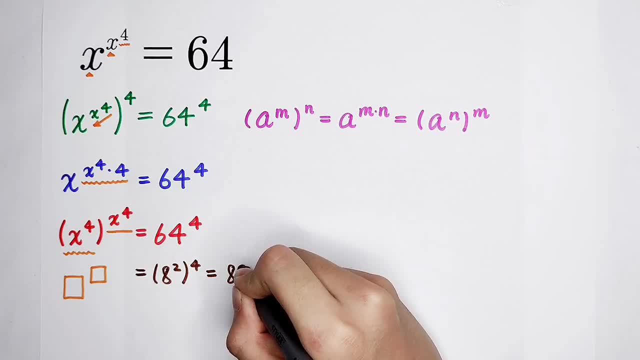 8 to the power of the product of 2 and 4.. It is equal to- Now it's enough, because 2 times 4 is 8. So it can be written as 8 to the power of 8.. Then 8 to the power of 8.